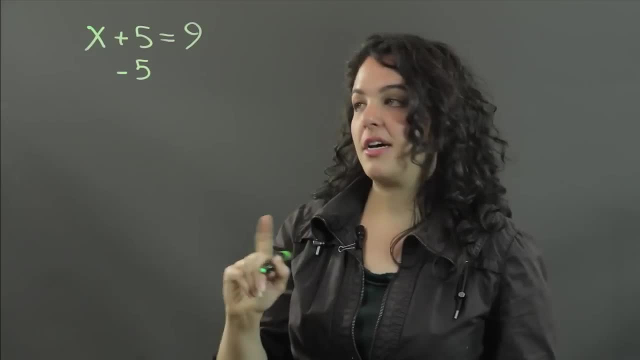 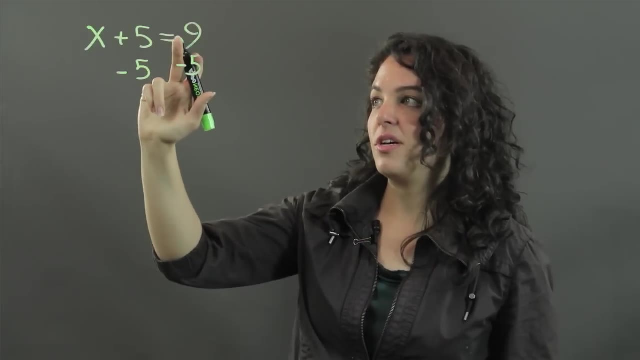 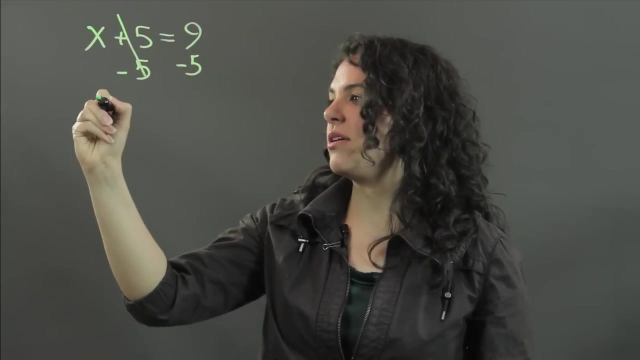 And we're going to subtract 5 from both sides. Whatever you do to one side, thou shalt do to the other side, in order to preserve the equality of each side. So when we subtract 5 from this side, these cancel out and we just get x, and 9 minus 5 is 4.. 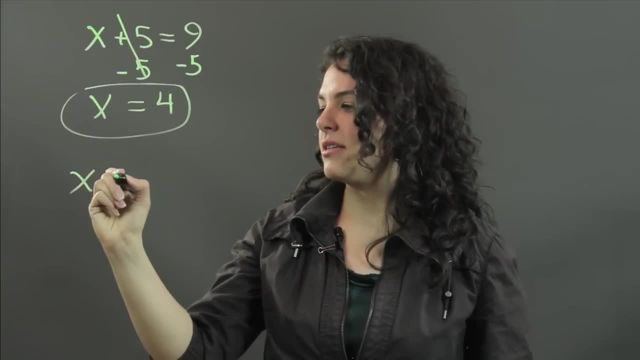 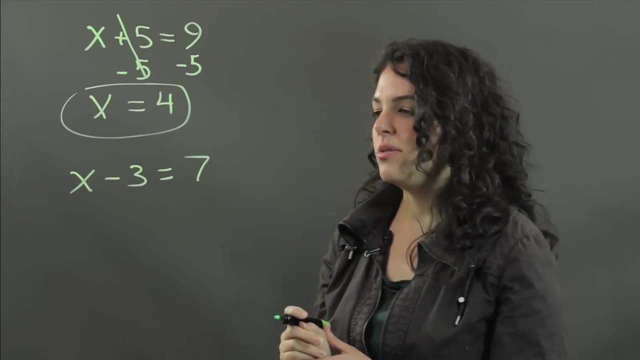 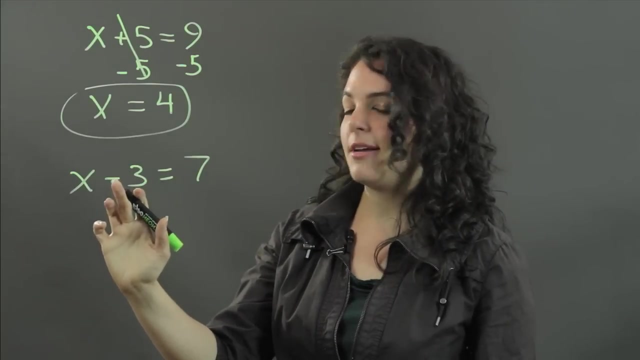 If you had another problem like: x minus 3 equals 7, we look at the operation between x and the number that we want to move over to the other side, which is 3 in this case, And we see that We are subtracting. 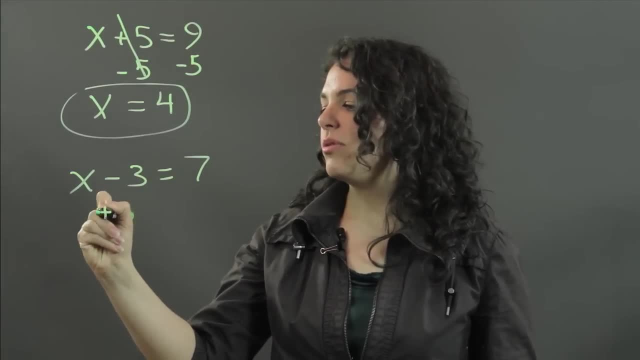 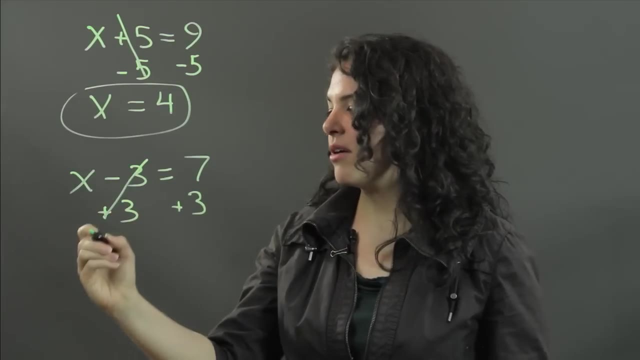 The inverse of subtracting is addition. We will add 3, again to both sides. Negative 3 plus 3 cancels out. We get x on this side And 7 plus 3 is 10.. x equals 10.. 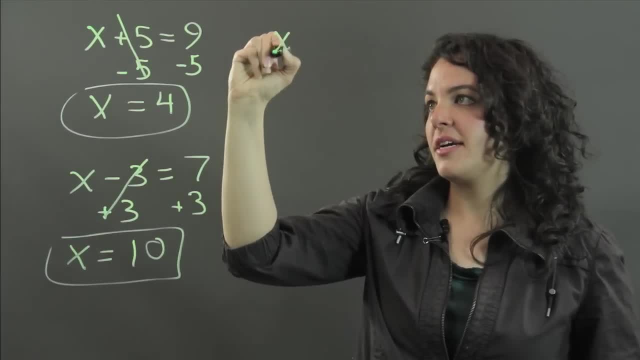 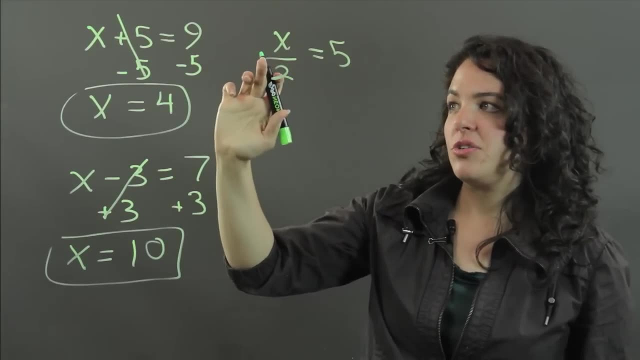 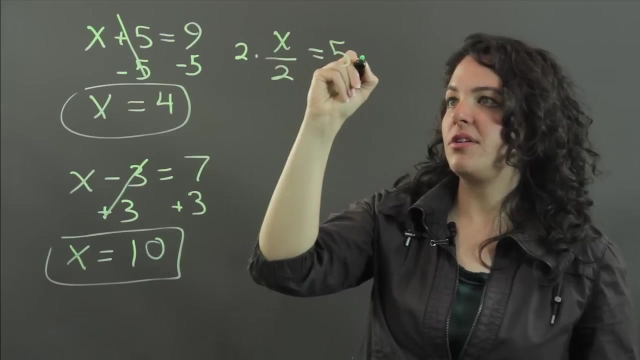 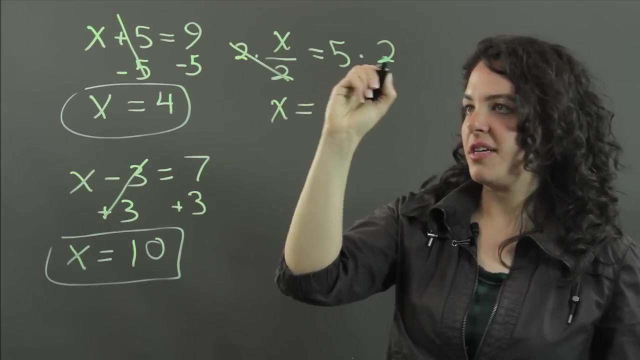 I'm going to give you two more quick ones. If I have x divided by 2 equals 5, x is being divided by 2.. The inverse of division is multiplication. So I'm going to multiply both sides by 2, multiply by 2, multiply by 2, 2 over 2 crosses out and I have x equals 5 times 2 is 10.. 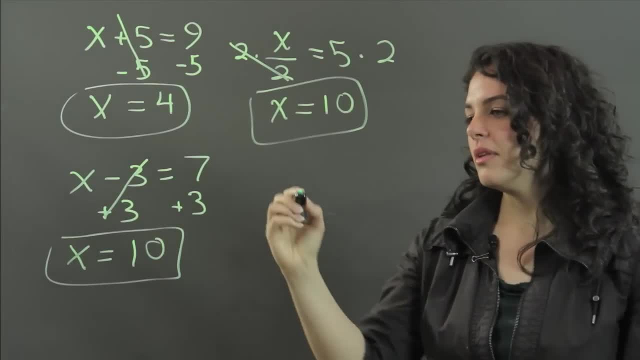 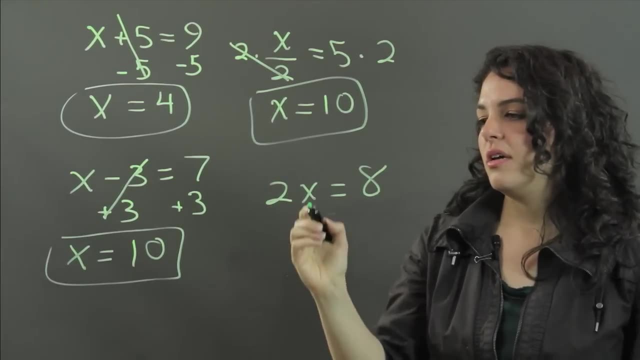 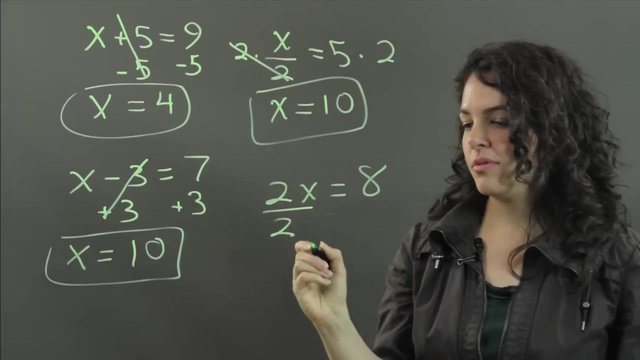 And then the last one: if I have 2 times x equals 8,, the inverse operation of multiplication is division. And then the last one: if I have 2 times x equals 8, the inverse operation of multiplication is division. So I'm going to divide by 2 from both sides. 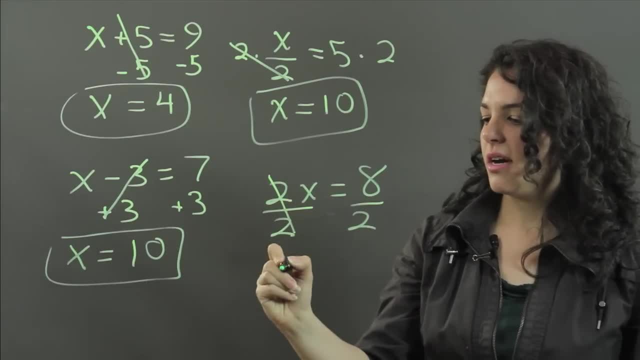 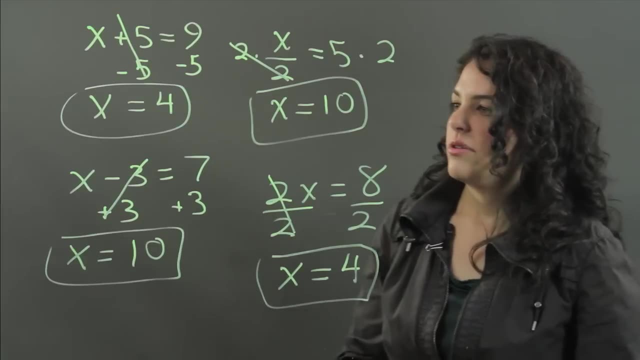 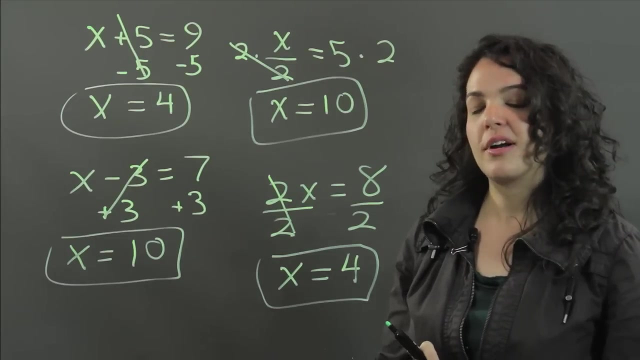 Remember that 2 over 2 cancels out. I get x equals 8 divided by 2 is 4.. So that's how you solve simple algebraic problems: using inverse operations, which will make the more complicated algebraic problems a lot easier, once you get the hang of this style. My name is Julia. Thank you, Thank you.